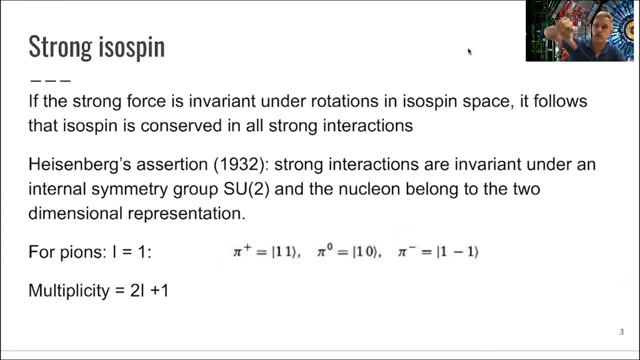 space. meaning when you flip the neutron into a proton and vice versa, those rotations are invariant. The strong force is invariant under those rotations. That means, or at least what follows directly, is that the isospin is conserved in all strong interactions. 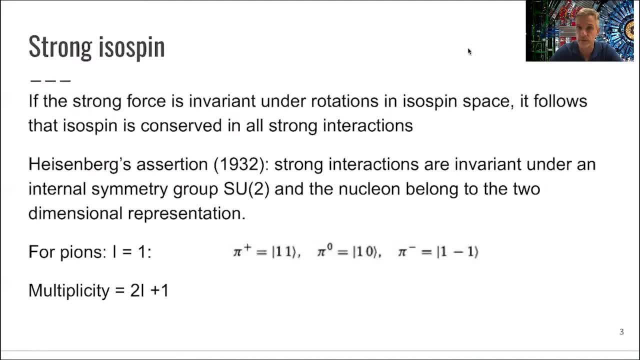 So that is what really the conclusion is of this introduction of those new labels, is that isospin is conserved under strong interactions. So this was proposed in the 1930s. Again, we notice the symmetry in nature and from that symmetry a conservation law follows Even so, and we can conclude: physics cross-sections. 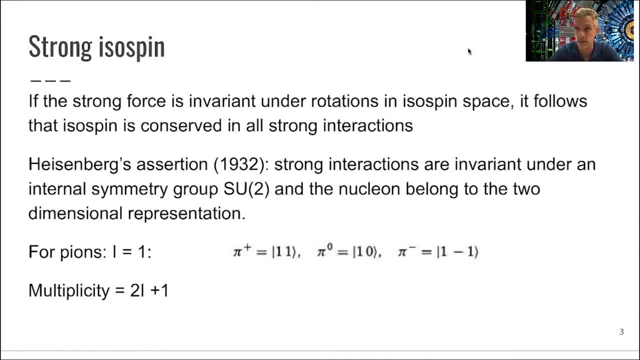 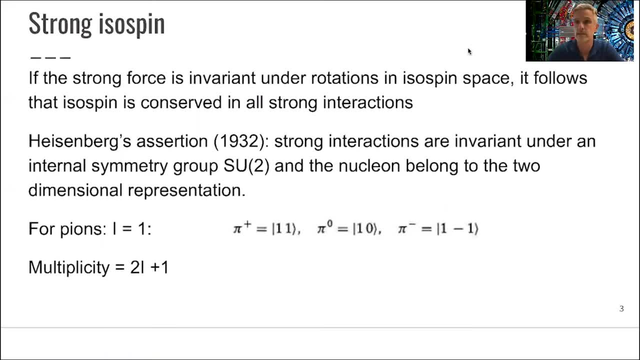 or ratios of cross-sections from it, without understanding, in this case, QCD use from interaction. But this is very fascinating and you can just apply this concept now to other particles, for example the pion. The pion has an isospin of 1, and there are three pions or three. 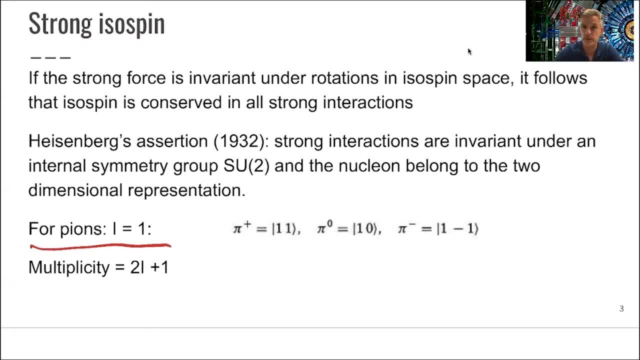 states: the zero state, the up state and the down state, which is the pi plus the pi zero and the pi minus. Well, you can conclude that the multiplicity of your particles, as you see, the neutron, the proton, the pi plus the pi zero and the pi minus, the multiplicity is 2 times. 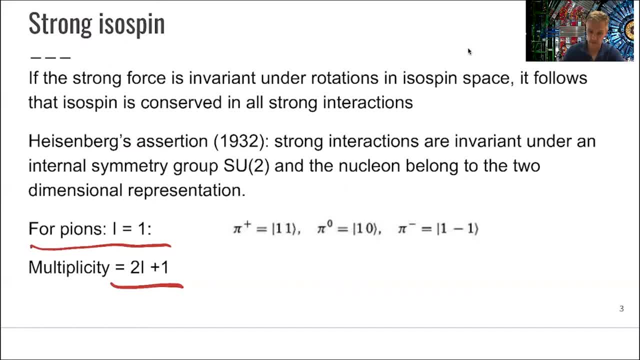 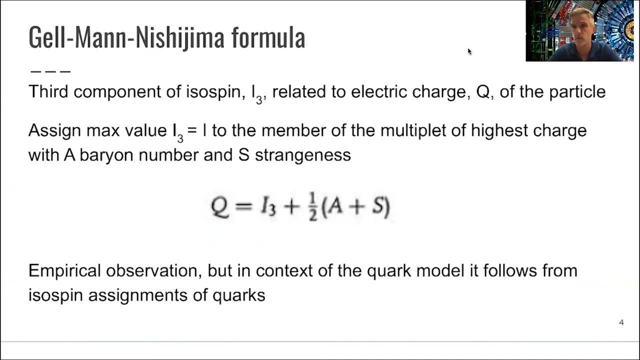 the isospin plus 1.. Isospin equal 1 means that there are three particles as part of the representation. So far, so good. So later this concept was, You know, Moved to other new particles. Many new particles were introduced and produced in the emergent accelerators and experiments. 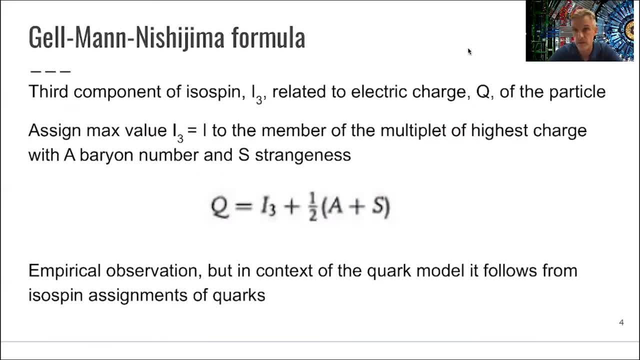 on the market and people tried to classify them in those By their isospin. Gell-Mann and Nishiyama empirically observed that there is a relation which holds this equation here, which is that the charge if you assign the maximum value. 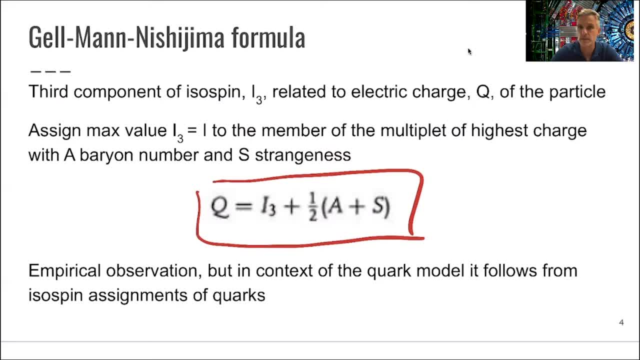 i3, the third component of your isospin to the member of the multiplet with the highest charge in the previous example was either the proton or the pi plus, then the charge of this particle follows from the isospin, the baryon number and the strangeness. 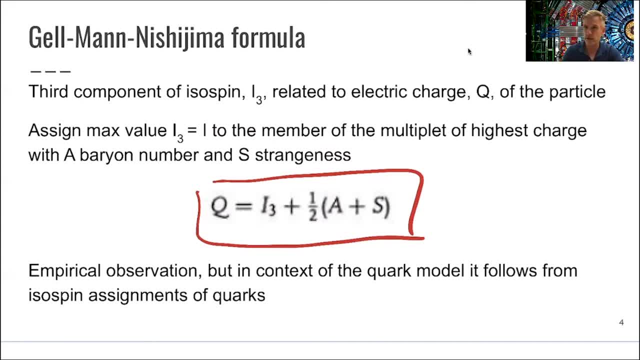 We looked at baryon number and strangeness before, but as a reminder, strangeness is the number of strange quarks in the baryon or the meson, and the baryon number is simply the number of baryons. 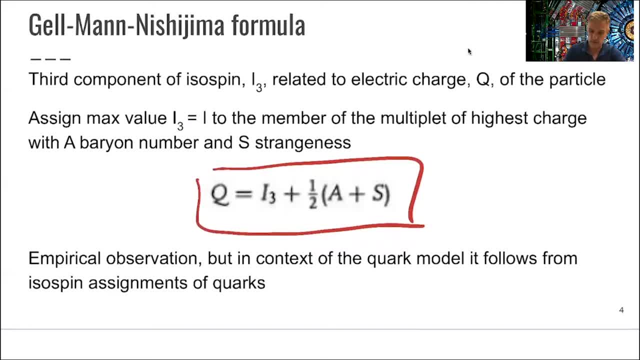 So if you just look at this, as for example for this pion case, we had the isospin equal one, baryon number equal zeros. strangeness equal zero, which follows that the maximum charge involved is one which is the charge of the positively charged power. 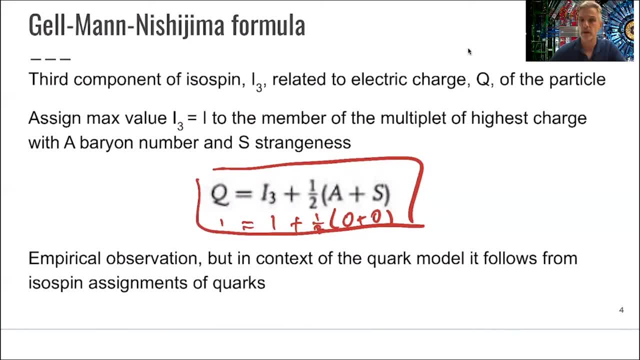 So far, so good. This was empirically observed, But once you then later discover, discover and develop a quark model, this is then in the 1970s- you can deduce this equation directly from the assignment of isospin to quarks, which is rather fascinating. 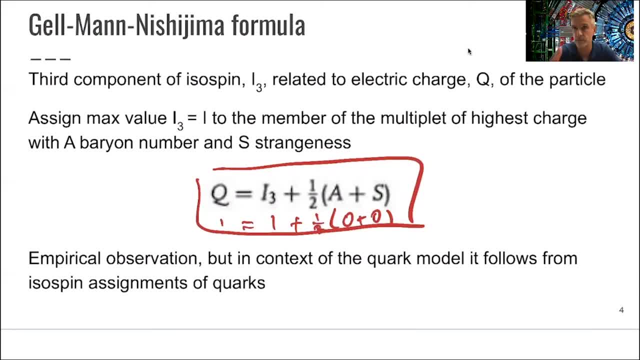 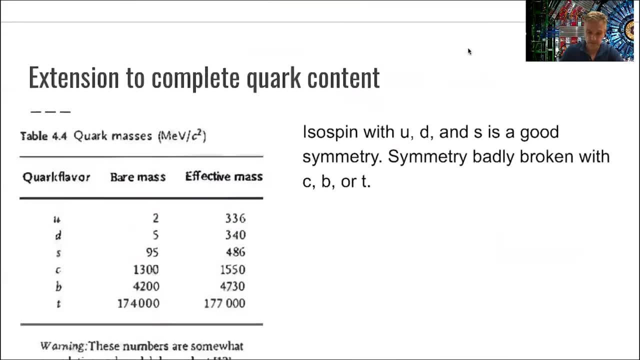 Again, you don't understand the physics fully, but just from the symmetry you can, and empirically you can, deduce information about physical systems. However, if you try to now extend this idea of isospin, you can deduce the number of particles. 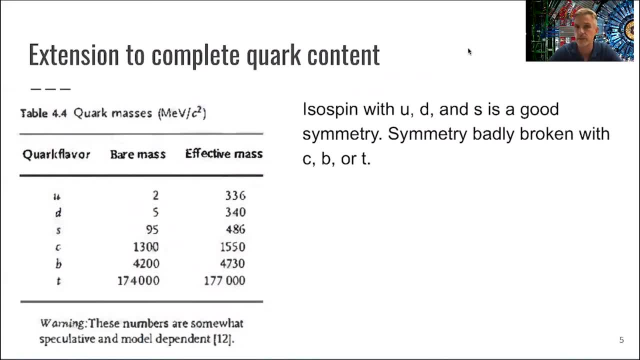 the idea of isospin to the complete quark model, you find that the symmetry starts to be broken. It already starts to be broken slightly when you include strangeness or strange quarks, but it's badly broken when you include charm bottom or top. 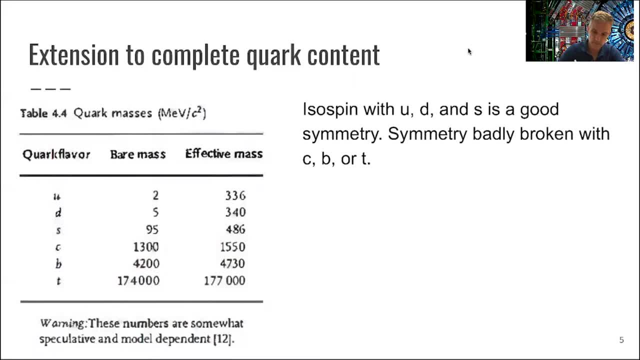 And the reason can be seen here: The up quark and the down quark, both of the particles making up ions, and the neutron and the proton, And even if you include strangeness, the difference in mass is not very large. So you know the symmetry. the particles you know really look like they're the same. 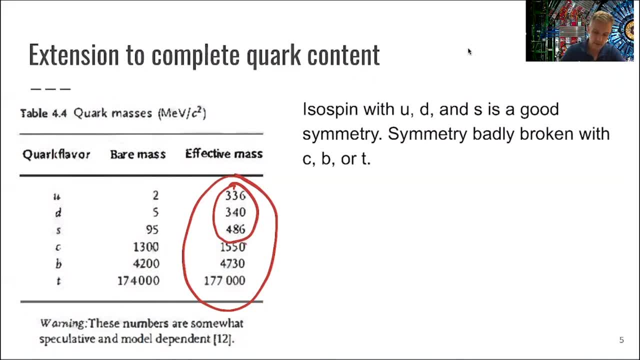 particle in a different state of the same particle. But when you introduce other quarks, heavier quarks, charm and bottom, you find that the mass differences are so large that the symmetries are broken. So this concept starts failing because of the large mass differences, because the symmetry 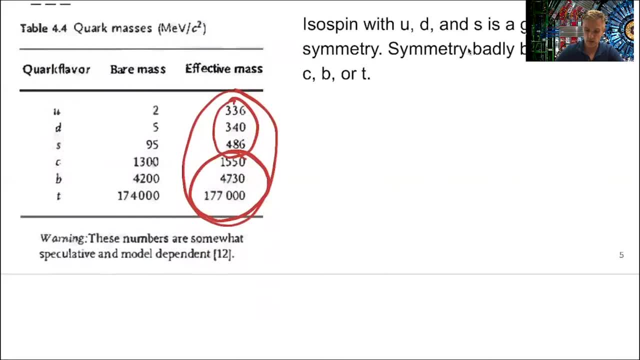 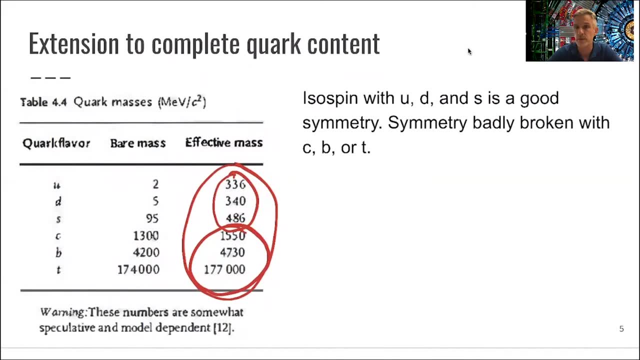 is broken, All right. so from here we now go to discrete symmetries, And again from the observation of those symmetries we can deduce physics without fully understanding the underlying physics.